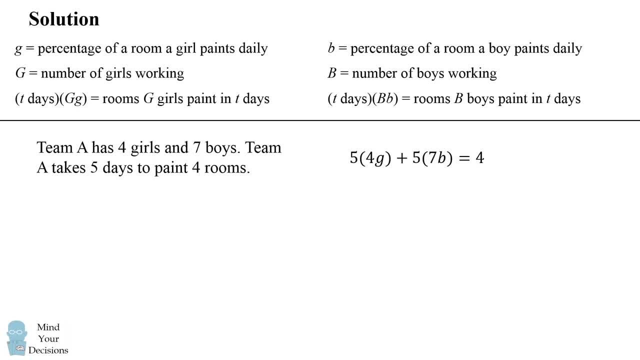 plus five times the quantity seven B is equal to four. Five times the quantity four G is the amount of work that the girls are doing, and five times the quantity seven B is the amount of work that the boys are doing to get a total of four rooms. 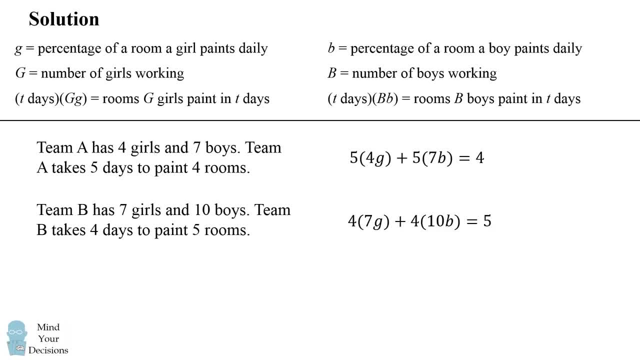 Now for team B. we can set up a similar equation: We have four times the quantity seven, G plus four times the quantity 10, B equals five. Now for team C. we know the number of girls and the number of boys and we know that there are six rooms. 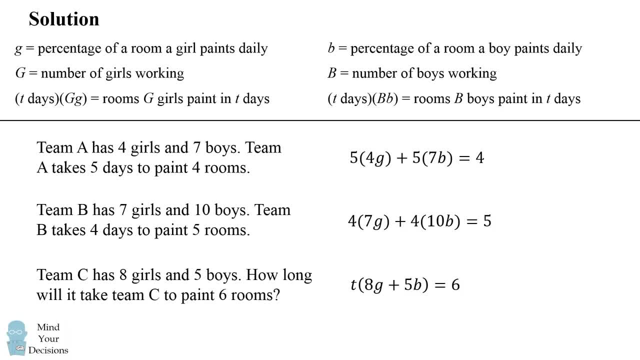 and we want to solve for the variable T. So we have T times the quantity eight G plus five B equals six. So how can we solve for T? Well, let's take a look at the first two equations we set up. We can rewrite the first equation as 20 G plus 30 B. 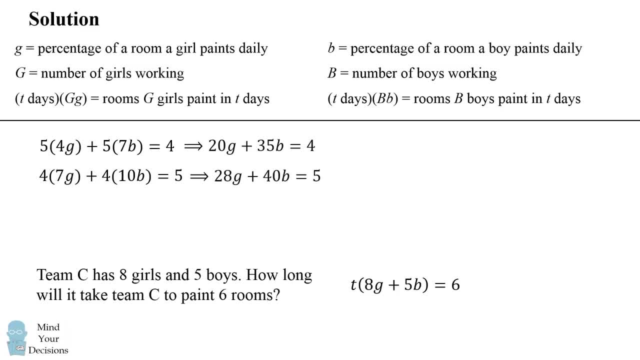 equals six. So we get 25. B equals four. The second equation becomes 28 G plus 40 B is equal to five. Now, if we subtract the first equation from the second, we get eight G plus five B is equal to one. 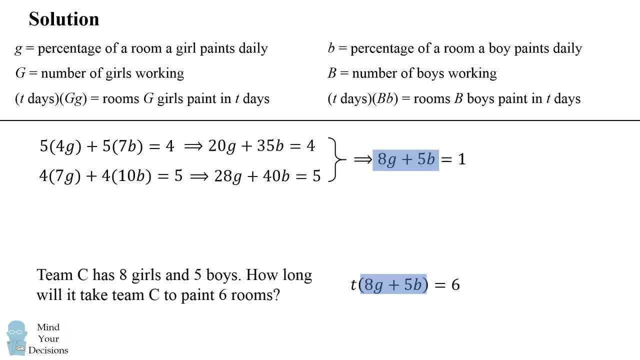 And that exactly matches what we want to find in team C. So just algebraically, if we multiply both sides by six, we can see that T has to be equal to six. But we can also interpret the answer If eight G plus five B is equal to one. 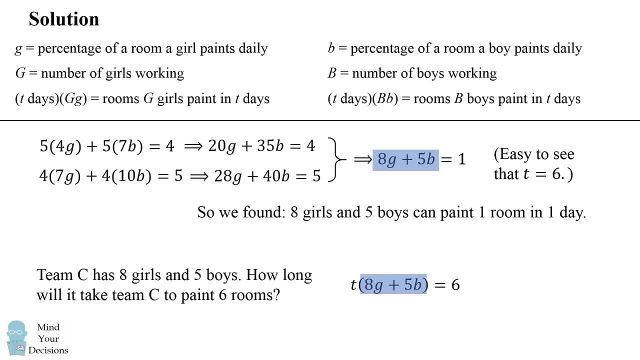 that means eight girls and five boys can paint one room in one day. Therefore, it will take six days for team C to paint six rooms. Did you figure it out? Thanks for watching this video. Please subscribe to my channel. I make videos on math. 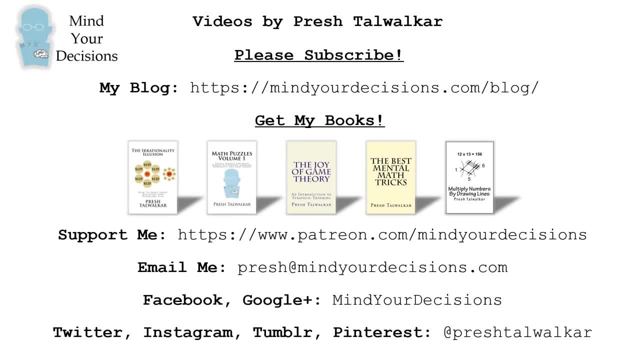 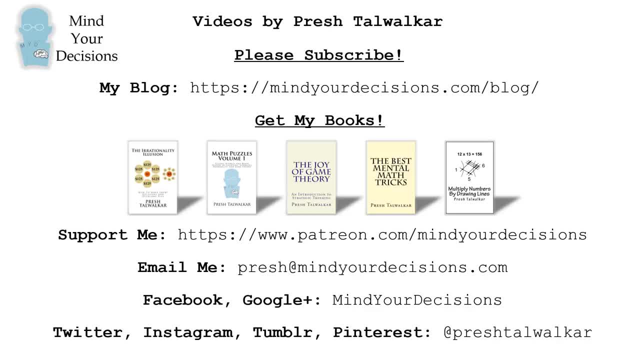 And you can catch me on social media either at mindyourdecisions or at preshtallwalker.